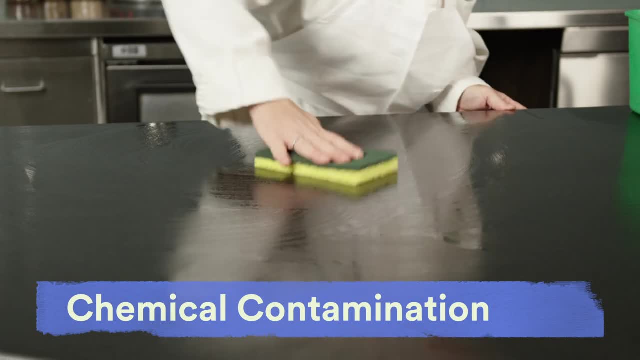 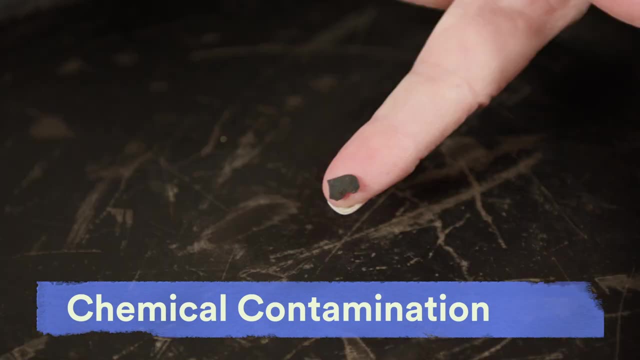 foods that are not in the food service industry. In a kitchen, chemical contamination can come from from the supplier, Cleaning compounds such as ammonia, chlorine or silver polish, Toxic metals or compounds used for cooking utensils such as chipped enamel or peeling Teflon. Physical 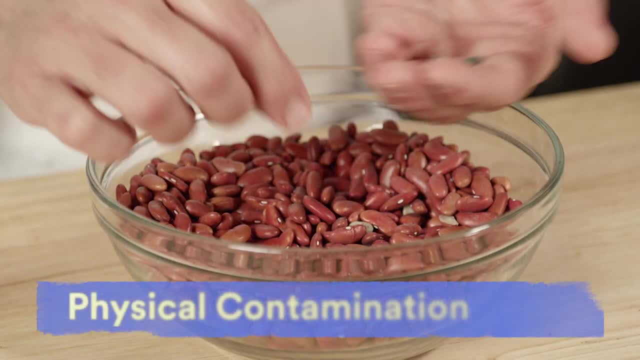 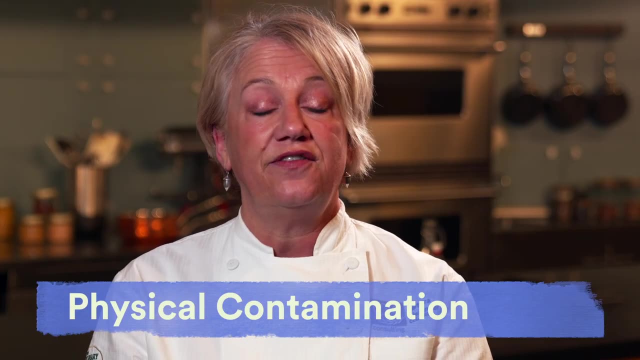 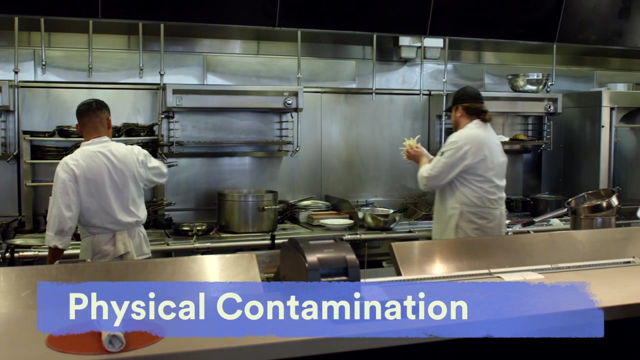 contamination can occur with the supplier or vendor, such as when foreign particles get into the food product during the harvesting or packing. More likely physical contamination occurs in the kitchen during food preparation and service, When hair, broken glass or splinters of wood or metal fall into the food. 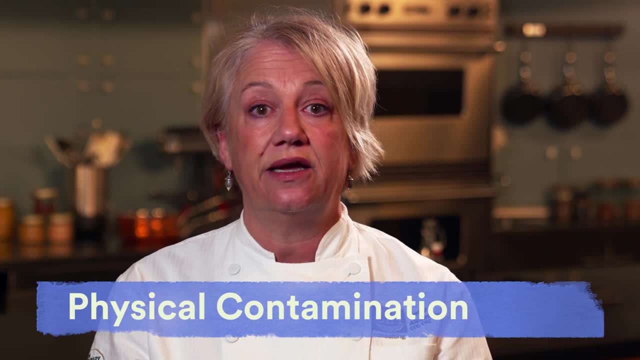 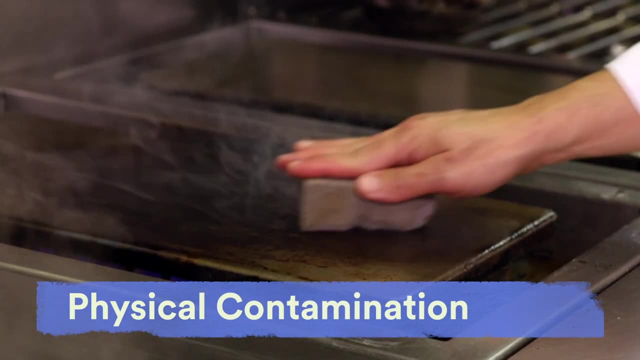 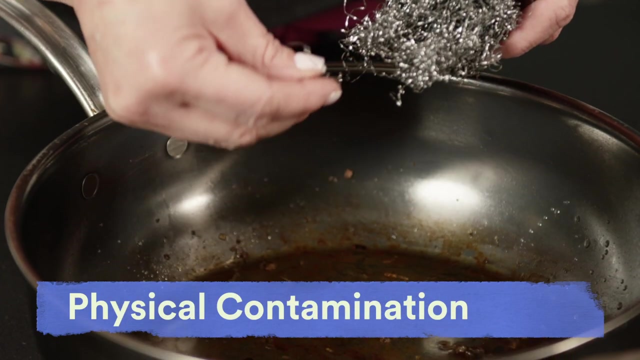 Physical contamination can also occur when cleaning. For example, scrubbing a griddle using an old or inferior quality grill brick can result in glass particles in the brick breaking off and getting into the food being cooked on the grill. Another example is when pieces of cleaning tools being 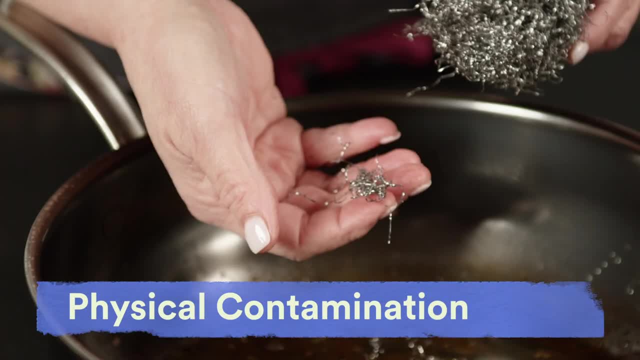 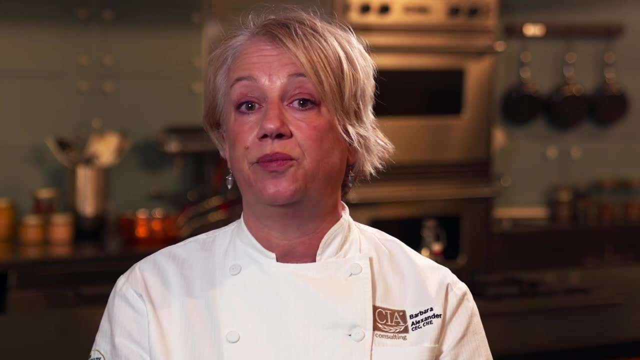 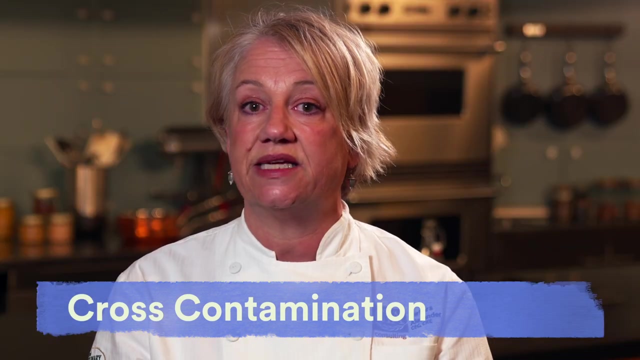 used to scrub pots and pans, such as pieces of metal from stainless steel. scrubbers contaminates the food being cooked. Cross-contamination is another danger during food preparation. This occurs when a previously safe item is exposed to an unsafe item and then becomes contaminated. The most obvious examples are in the use of cutting boards. 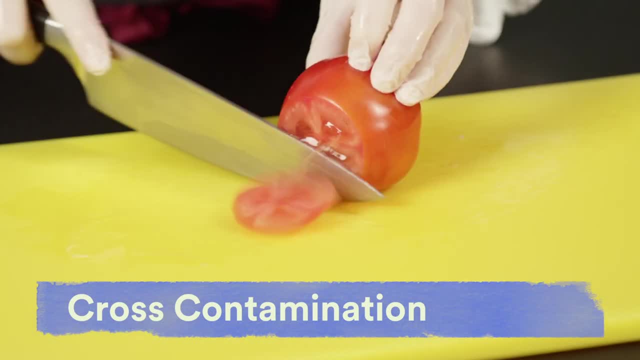 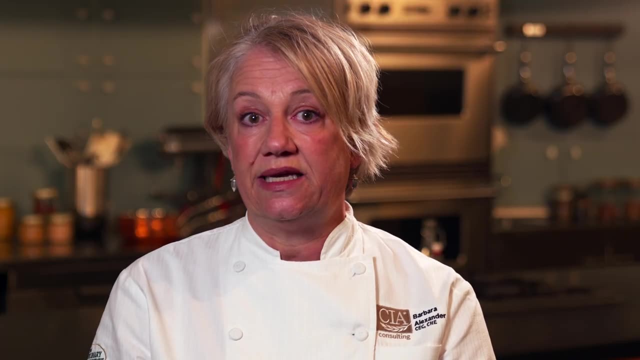 If you have just placed raw chicken on a cutting board, you don't want to cut your tomatoes for the salad on that same cutting board. Now that we've talked about how foods can become contaminated, in the next video we'll talk about what you should do to prevent food contamination. 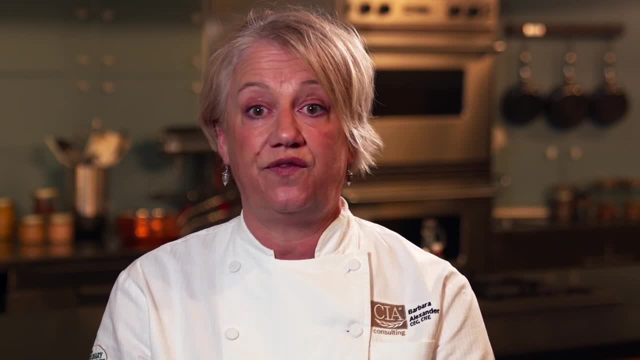 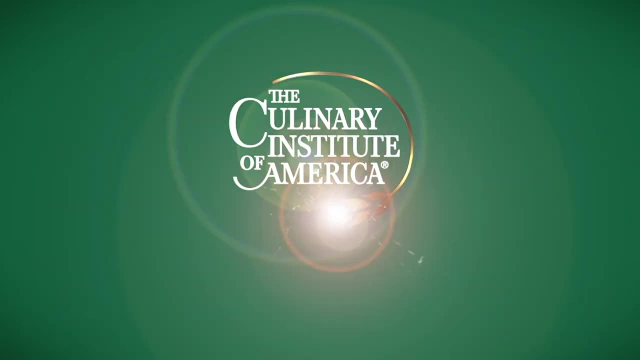 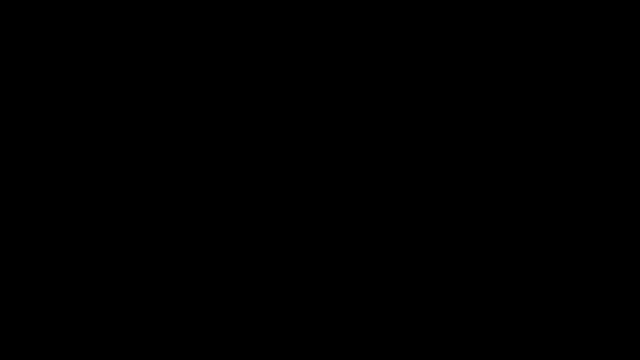 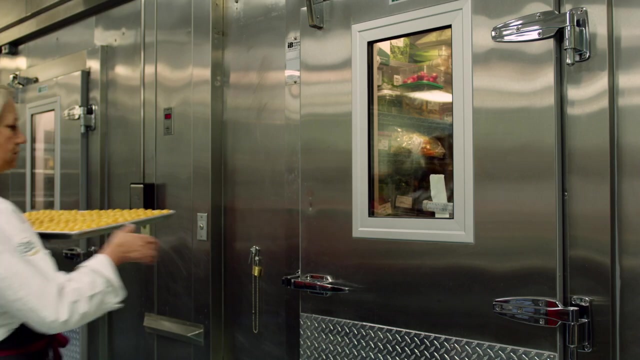 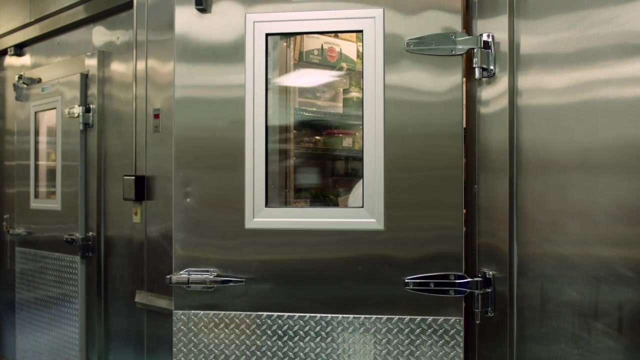 We'll talk about what we can do in the kitchen to keep foods and our customers safe. We'll talk about what we can do to prevent food contamination. We'll talk about what we can do to prevent food contamination. We'll talk about what we can do to prevent food contamination. 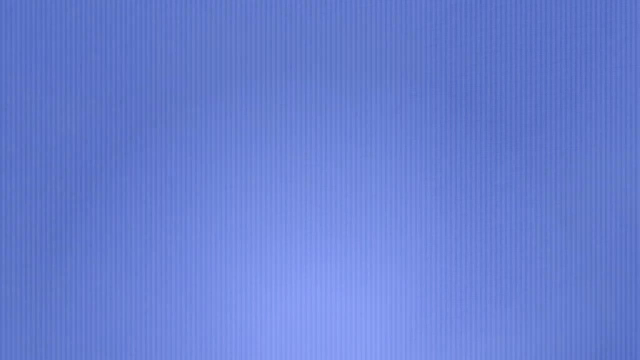